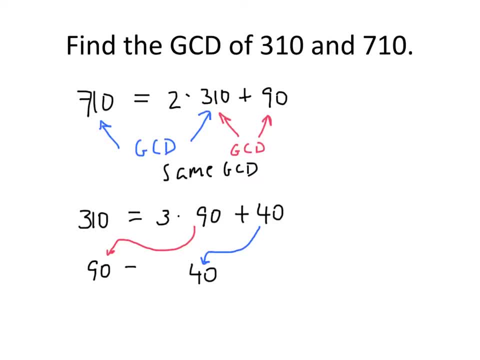 So the 40 moves over here. And now we're going to take 90 and divide it by 40. 40 goes into 90 twice, remainder 10. One more time, as we'll see. The old divisor becomes the new dividend. The old remainder becomes the new dividend. The new divisor. And 10 goes into 40 four times, remainder 0. And 0 is our signal to stop. 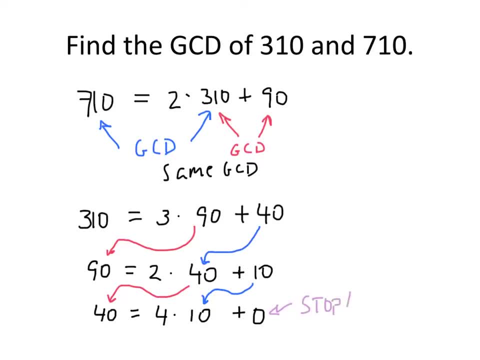 Once we get a 0 remainder, that's when we stop this process. And the reason is because, again, the two numbers that we're dividing, in this case at this last step, we divided 40 by 10. Well, the greatest common divisor of 40 and 10 is the same as the greatest common divisor all the way back at the beginning that we were looking for. So the greatest common divisor has not changed at all at any of these steps. And if we were to go one more step, then we would be looking at the greatest common divisor of 10 and 0. 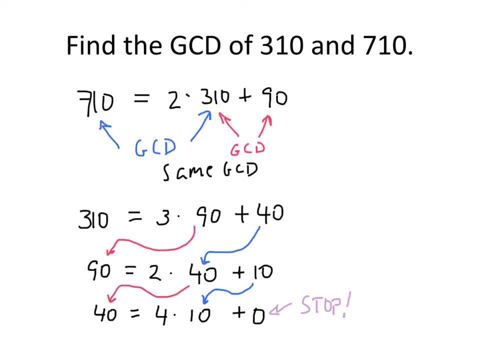 But everything divides 0. 0 is divisible by everything. 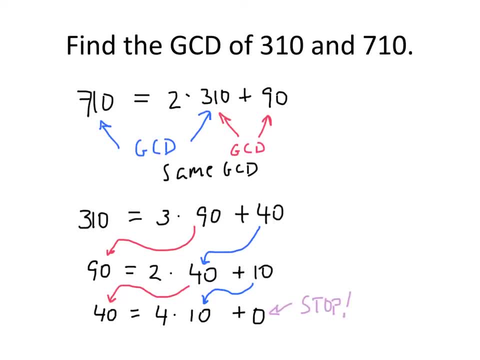 So the greatest common divisor of 10 and 0 is really just the greatest divisor of 10. 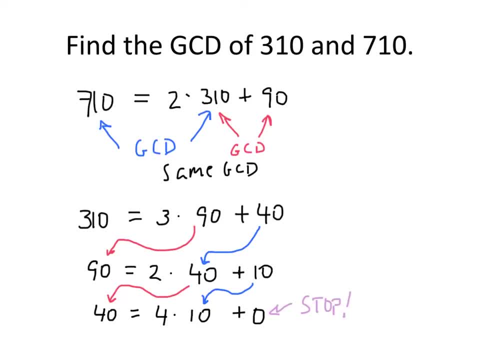 And the greatest divisor of 10 is 10. So that means that the greatest common divisor is equal to 10. 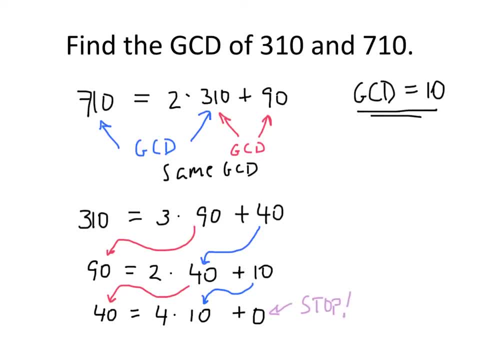 In practice, what this means is that the last non-zero remainder, which is this 10 right here, that's your GCD. The last non-zero remainder. 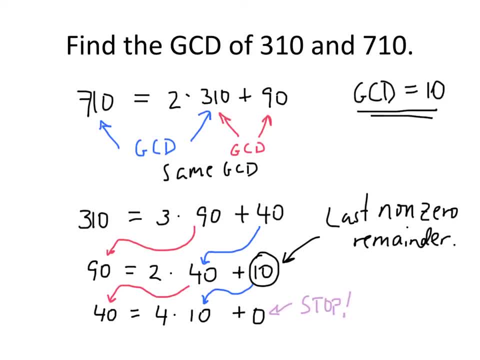 So the Euclidean algorithm for finding the GCD has us repeatedly dividing. And at each step, the new dividend, follow these red arrows, the new dividend is the old divisor. And the new divisor, following these blue arrows, the new divisor is the old remainder. So we keep shifting these numbers to the left until we get to a 0 remainder. 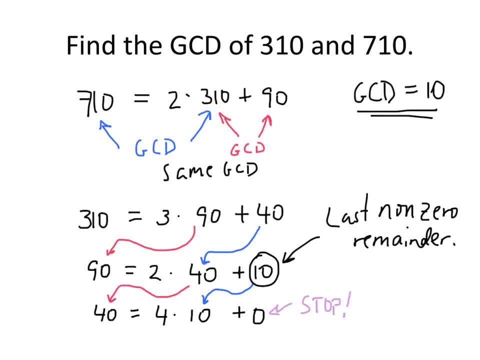 Once we get a remainder of 0, and we will always get a 0 remainder at some point, the remainders are always going to get smaller and eventually they have to go down to 0. Once that happens, the last non-zero remainder, that's your GCD.